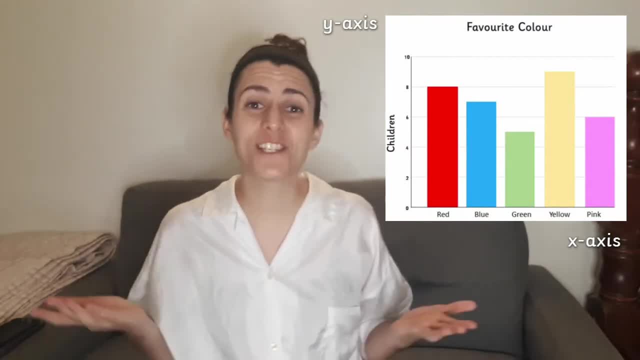 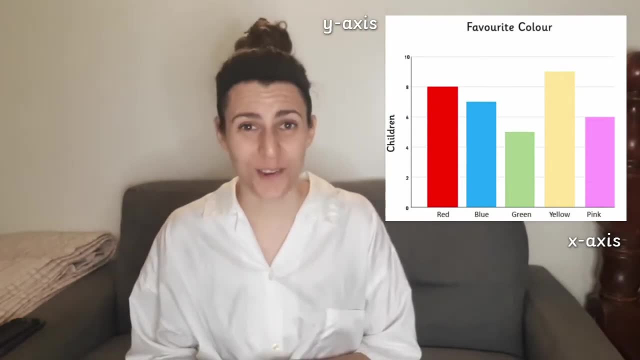 falls between the two numbers given. In our example, there are five children who chose green, because the bar aligns with the gap between four and six. So do all bar charts look like this? No, There are a few different ways data can be organized in a bar chart. Let's go through some. 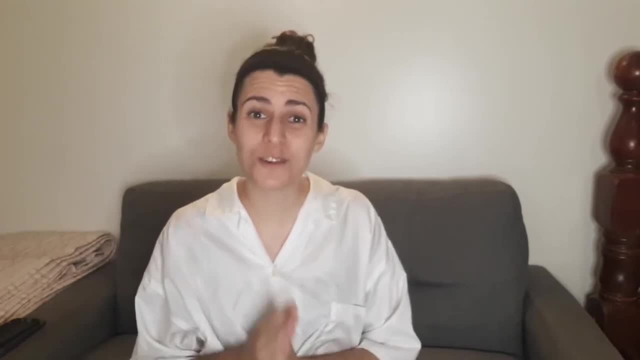 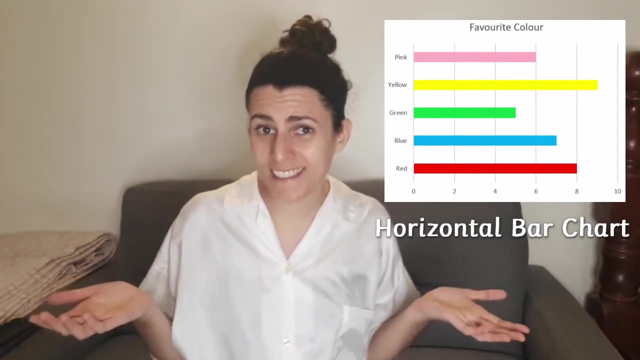 of them briefly. Our previous example was a vertical bar chart, but you can also get horizontal bar charts. These are pretty much exactly the same, just lying on their side. Maybe our bar chart got a little sleepy and wanted to lie down for a bit, Or maybe a horizontal bar chart would. 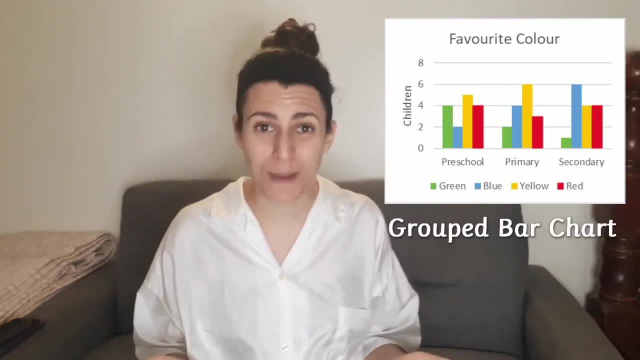 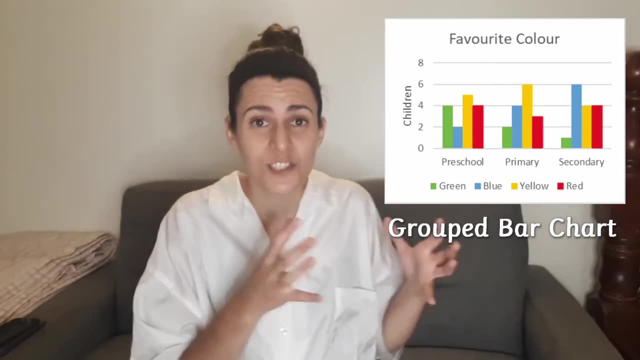 just fill the space in your document better. You can also get grouped bar charts. Sometimes, when you're making a bar chart, you may realize that the information cannot only be separated into categories but into groups within them. In this example, we are still looking at the popularity. 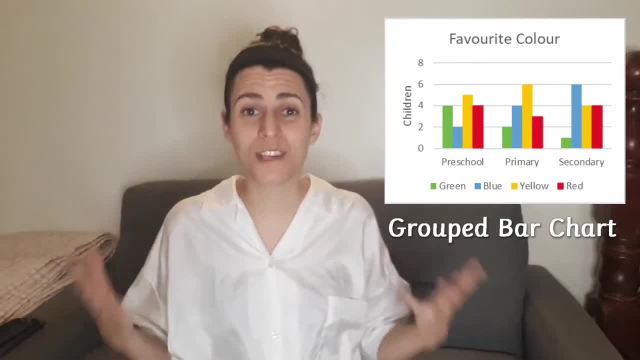 of different colors our categories, but have also grouped them into broad age groups depending on their year of schooling. This is handy because you can see that there are a lot of different categories in the bar chart. You can also see that there are a lot of categories in the bar chart. 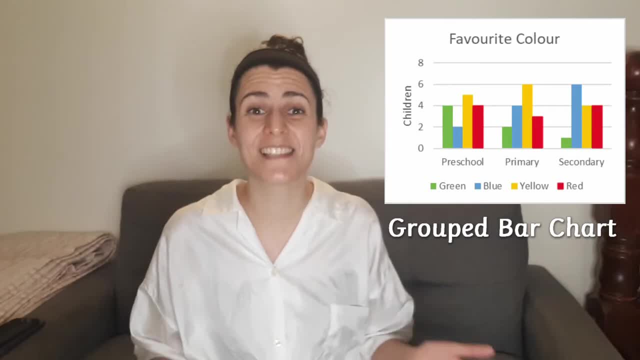 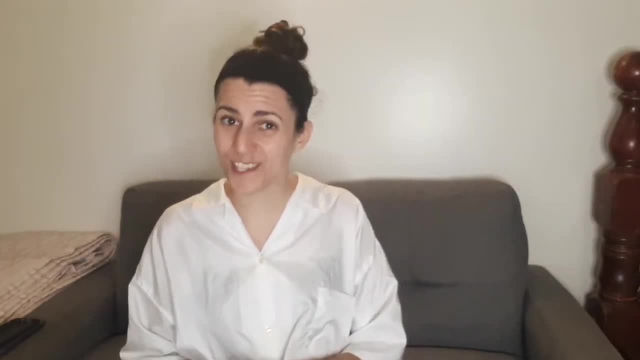 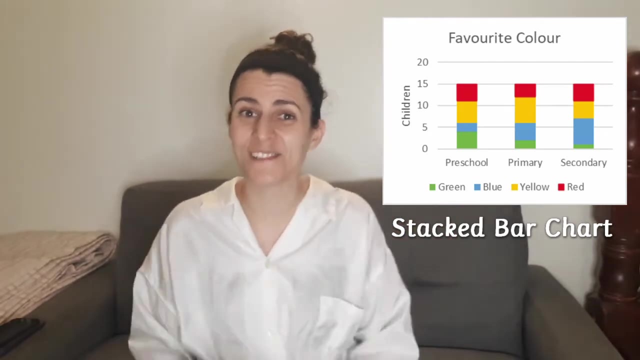 compare the categories, but groups within them as well. You can also get stacked bar charts. These are pretty much exactly the same as grouped bar charts, except instead of the bars sitting neatly next to each other, they're stacked on top of each other. This is helpful because each stack represents 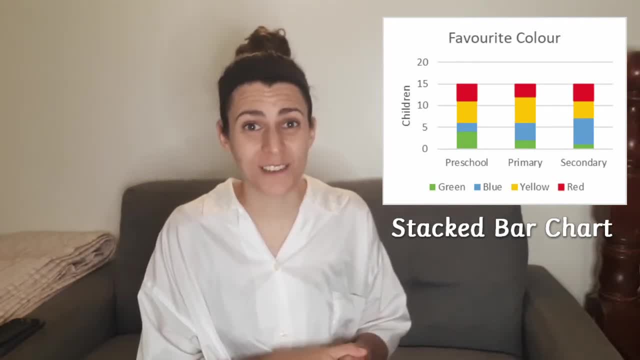 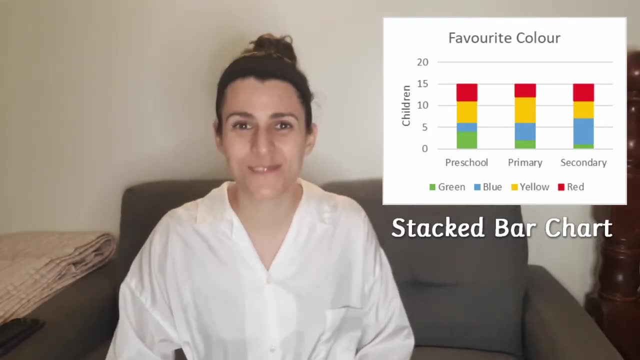 one whole, so you don't need to do any adding up to figure out its value, Like in our example, you can easily just look at it and tell that there were 15 children who were polled in each age group. Boom, Too easy. You can also get clustered, stacked bar charts. This is a mix of a grouped bar chart. 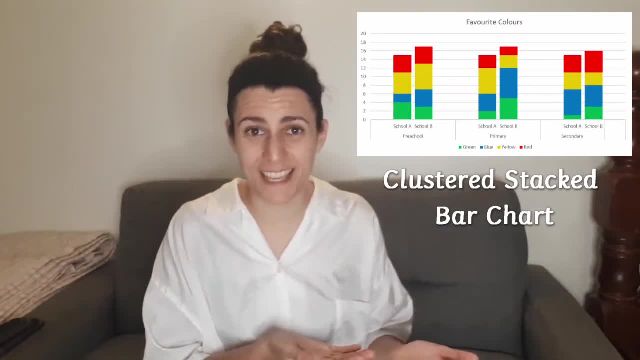 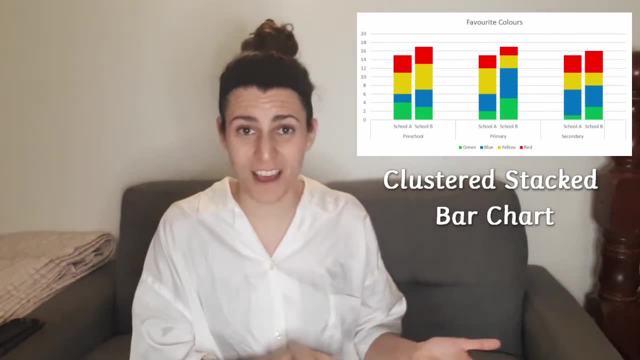 and a stacked bar chart, because we're taking stacks and grouping them together, Just like in this example. This lets you break down the data even further. Like here, we are not only comparing favourite colours among age groups, but also schools. So I get that seeing all these different. 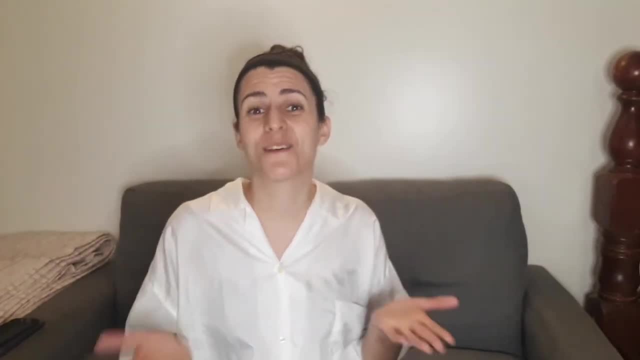 kinds of bar charts can be a little overwhelming, but it's handy to know, because when you're deciding what kind of bar chart you want to use to represent your data, you can think about your goals and your goals, and then you can decide what kind of bar chart you want to use to represent. 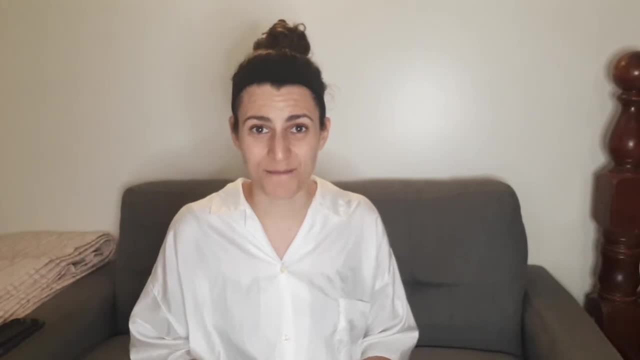 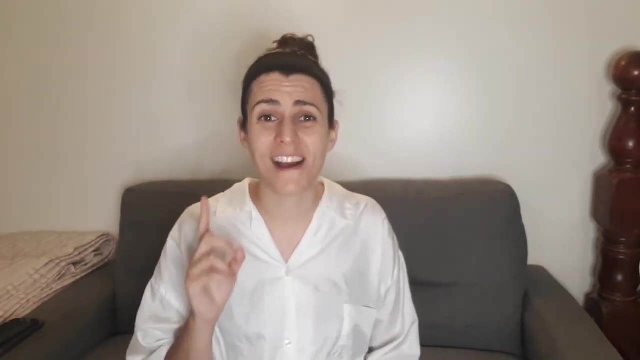 your goal and what you're trying to achieve, and then choose the most appropriate one. Overall, there are many reasons why we might use bar charts to organise our data. One reason is that it makes it really easy to compare our different categories. Looking at some of our earlier examples, 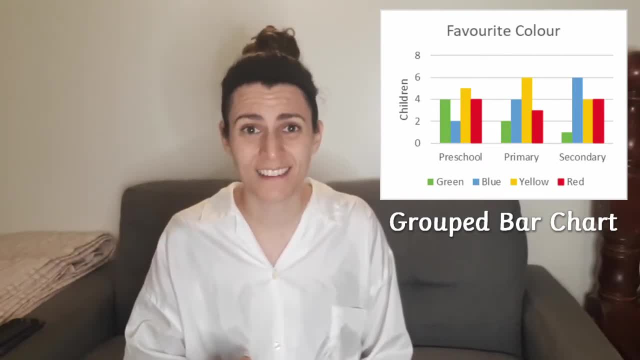 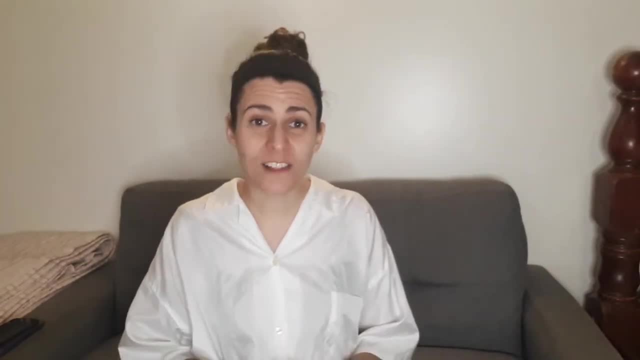 you can see right away that yellow is a very popular colour because it has the highest number of children liking it. They also make it easier to see trends and patterns in data. If the value of a category is growing or shrinking, this is called a trend. A pattern is something that seems to keep. 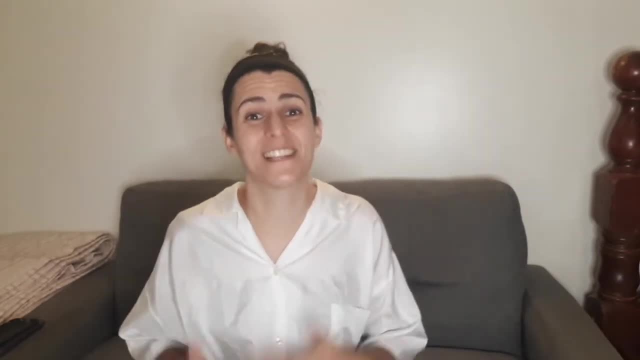 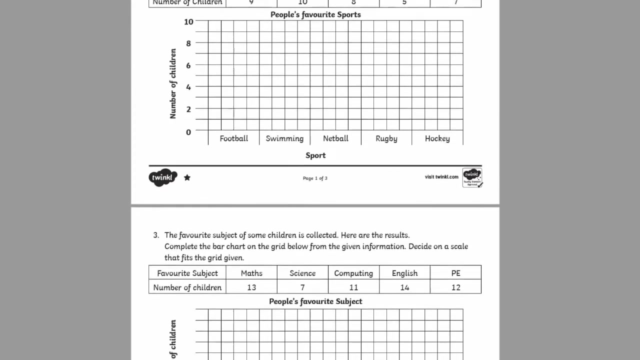 happening. Laying out this data so you can interpret your patterns and trends is one of the benefits of bar charts. Luckily, Twinkl has a great range of educational resources for learning about bar graphs. For instance, these differentiated worksheets have activities that give learners practice making bar charts using given data. The activities build on each. 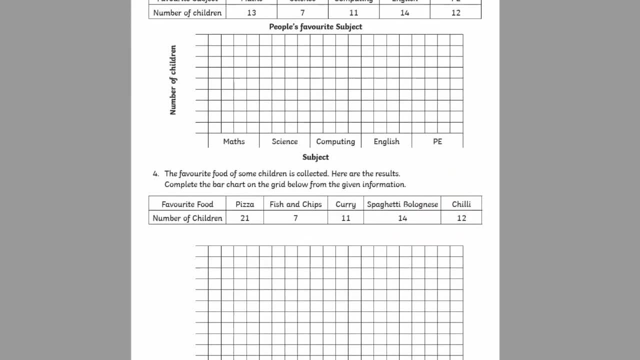 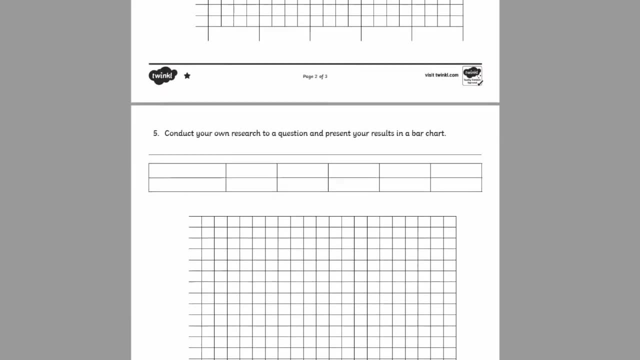 other to ease you in, so you can go from completing a partially completed bar chart to making your own from scratch. And, as I mentioned, they are differentiated, so learners can have a go at the option that suits them and challenges them appropriately. Of course, there are plenty of. 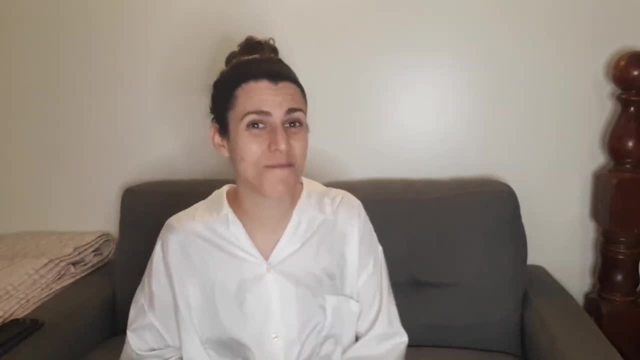 other helpful materials available on the Twinkl website, so make sure you have a browse and see what's out there. That's all for now, but thank you so much for watching and I hope you have a lovely day. 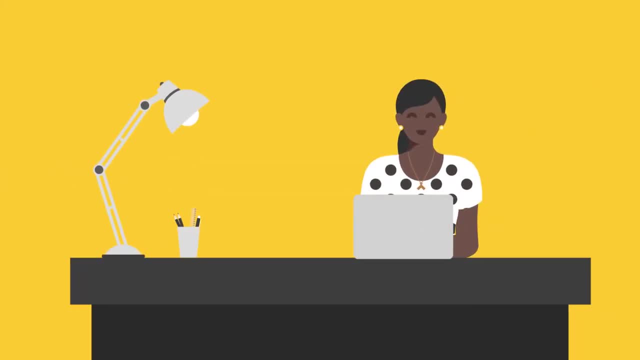 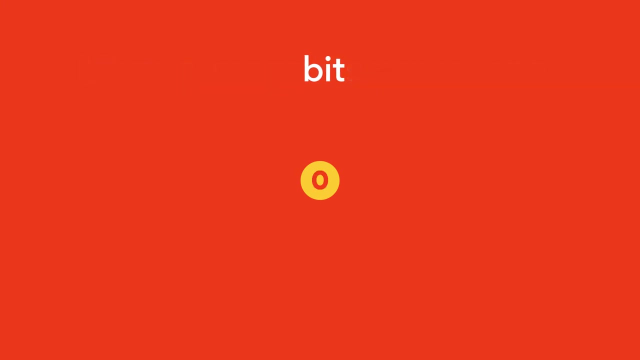 Shopping around for internet, You've probably noticed that plan speeds are measured in MBPS. But what are MBPS and how many do you need? MBPS stands for megabits per second. A bit is a tiny piece of data and a megabit is many, many tiny pieces of data, Not to be confused with megabytes. 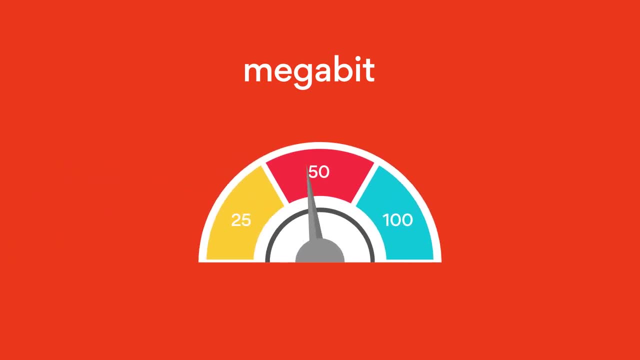 Megabits are what is used to measure your download speed. The higher the number of megabits, the faster your internet will be. So how many megabits per second do you need? Checking emails and browsing the internet usually uses only a small amount of data. A little more data is needed. 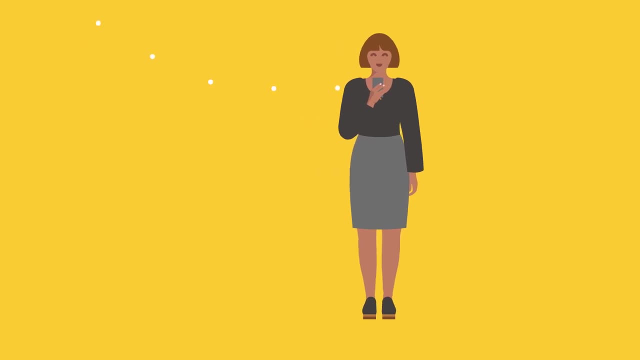 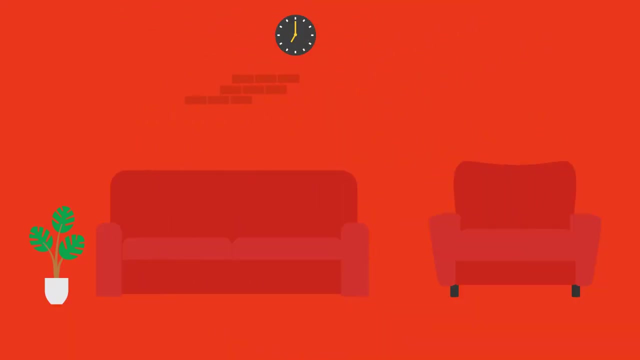 for apps like FaceTime or Skype. If you stream TV shows, download big movie files or watch live sport, you'll be using a whole lot more data, And if everyone in the house is internet streaming, gaming and everything in between, you're going to need more megabits per second to keep everyone.